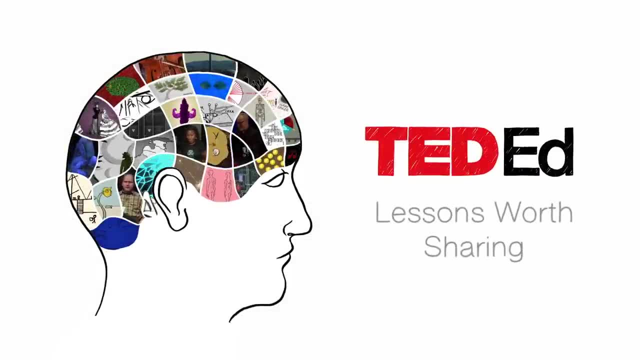 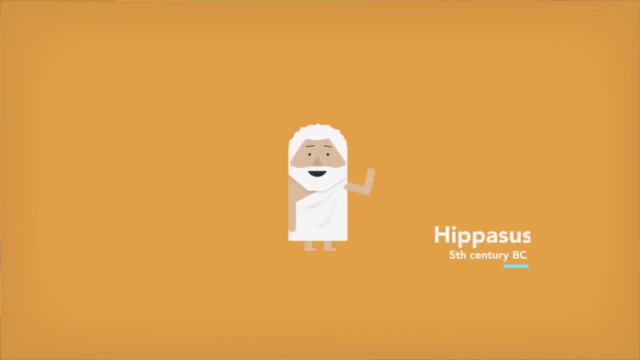 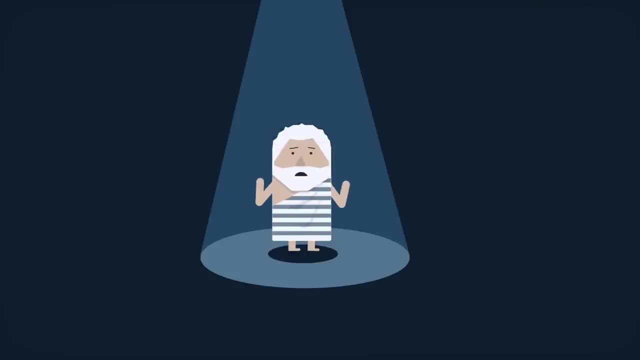 Like many heroes of Greek myths, the philosopher Hippasus was rumored to have been mortally punished by the gods. But what was his crime? Did he murder guests Or disrupt a sacred ritual? No, Hippasus' transgression was a mathematical proof. 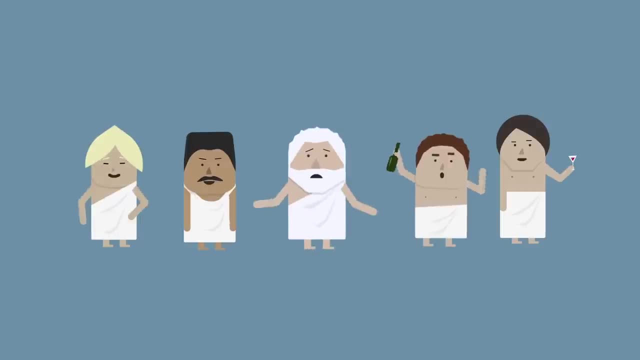 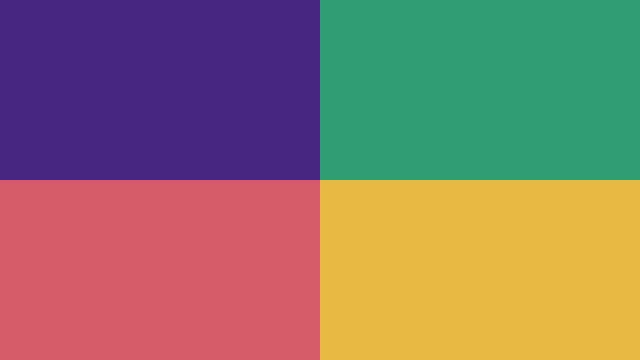 the discovery of irrational numbers. Hippasus belonged to a group called the Pythagorean mathematicians, who had a religious reverence for numbers. Their dictum of all is number suggested that numbers were the building blocks of the universe, And part of this belief was that everything from cosmology and metaphysics 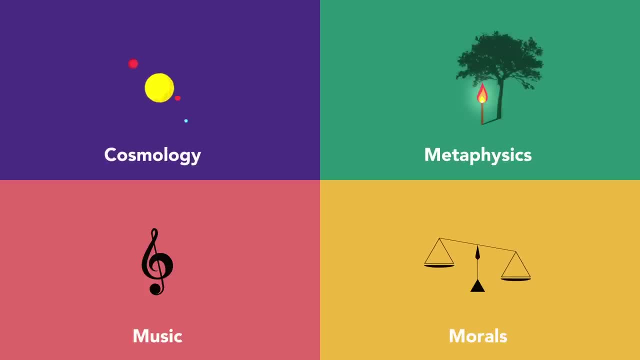 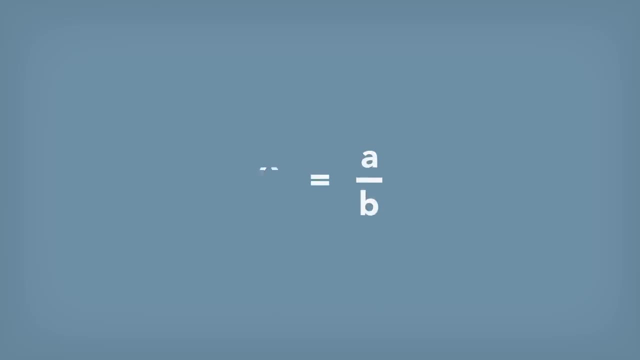 to music and morals followed eternal rules describable as ratios of numbers. Thus, any number could be written as such a ratio: 5 as 5 over 1,, 0.5 as 1 over 2, and so on. 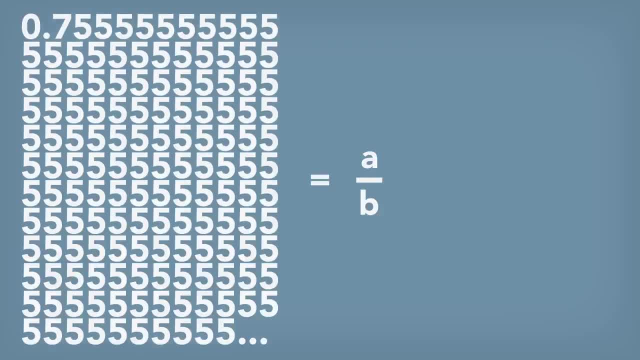 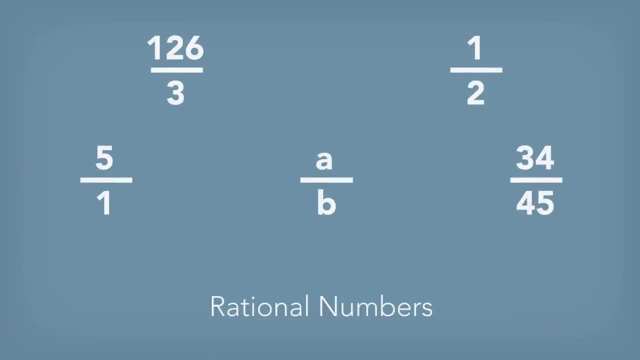 Even an infinitely extending decimal like this could be expressed exactly as 34 over 45.. All of these are what we now call rational numbers, But Hippasus found one number that violated this harmonious rule, one that was not supposed to exist. 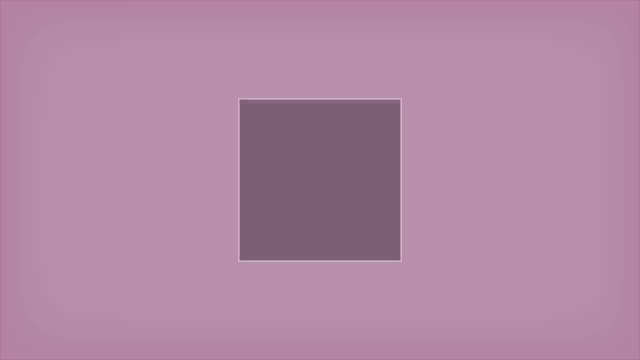 The problem began with a simple shape, a square, with each side measuring one unit. According to Pythagoras' theorem, the diagonal length would be square root of 2, but, try as he might, Hippasus could not express this as a ratio of two integers. 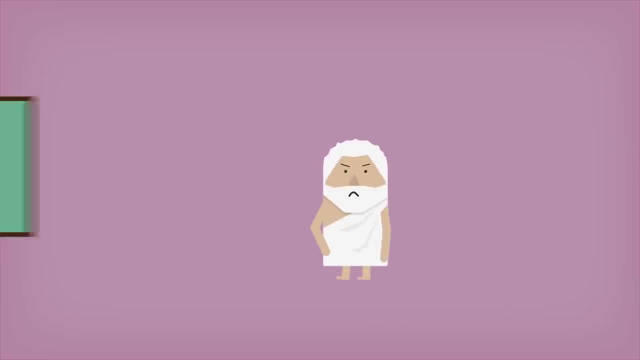 And instead of giving up he decided to prove it couldn't be done. Hippasus began by assuming that the Pythagorean worldview was true, that root 2 could be expressed as a ratio of two integers. He labeled these hypothetical integers p and q. 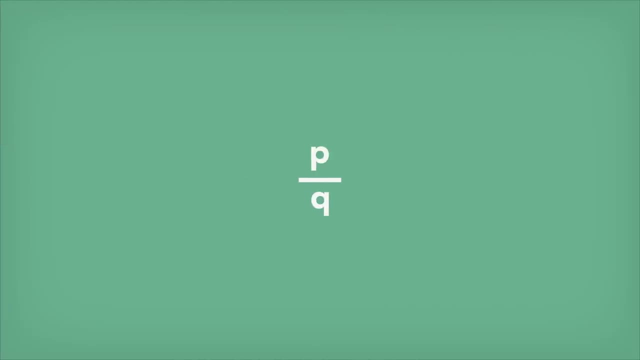 Assuming the ratio was reduced to its simplest form, p and q could not have any common factors To prove that root 2 was not rational. Hippasus just had to prove that p over q cannot exist. So he multiplied both sides of the equation by q. 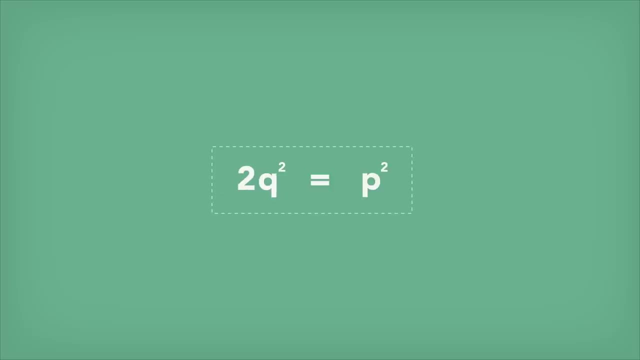 and squared both sides, which gave him this equation: Multiplying any number by 2 results in an even number, so p squared had to be even. That couldn't be true if p was odd, because an odd number times itself is always odd.